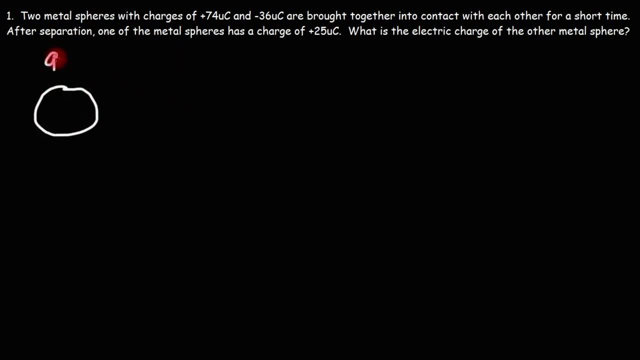 let's draw two pictures. We'll say this is charge one, Charge one, initial. so that's before contact. and here's another metal sphere. we'll call it charge 2, initial. Charge one has a positive charge of the 74 microcoulombs and charge two: 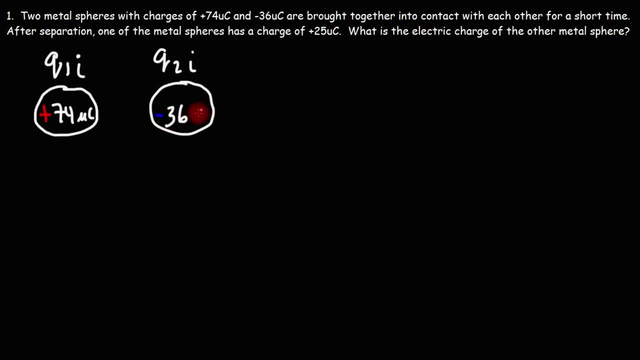 it's negatively charged and its 36 microcoulombs. Now, after contact, we have the charge of one of the metal spheres. let's say charge one, it really doesn't matter which one. so we'll call this q1 final, and it has a charge. 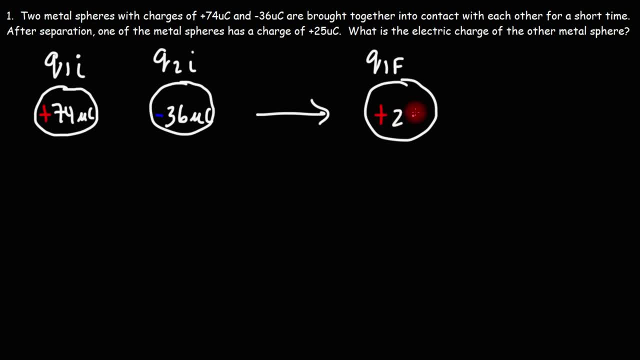 of positive 25 microcouples. what is the charge of the other metal sphere after contact? what's q2 final? well, according to the law of conservation of electric charge, the total charge Q initial be before contact was made- must equal the total charge after the two metal spheres came into contact with each other. since 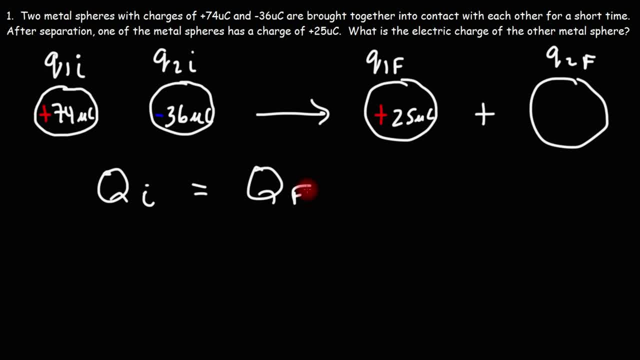 this is the closed system. there's no outside forces after. on this system the total charge before and after contact must be the same. so the total charge before contact is the sum of q1 initial and q2 initial. the total charge after contact is the sum of q1 final and q2 final. so q1 initial is. 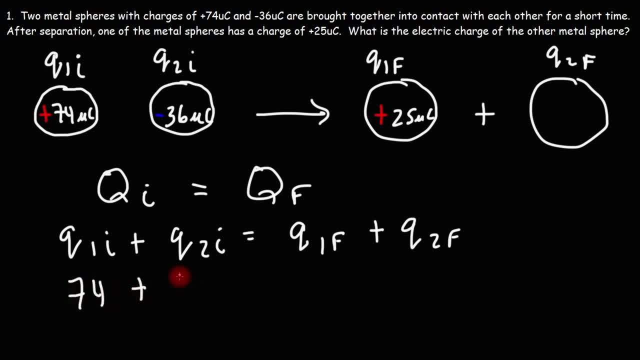 positive 74. q2 initial is negative 36. q1 final is 25. and now we got to solve for q2 final: 74 minus 36, that's 38, and if we subtract both sides by 25, 38 minus 25 is 13. 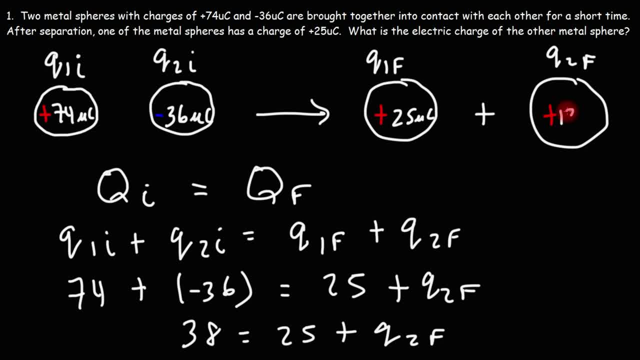 so the charge, the electric charge on the other metal sphere, is positive 13 micro coulombs. so if you add up 74 and negative 36, you get 38. that's the total charge before contact was made and after 25 plus 13. that's also. 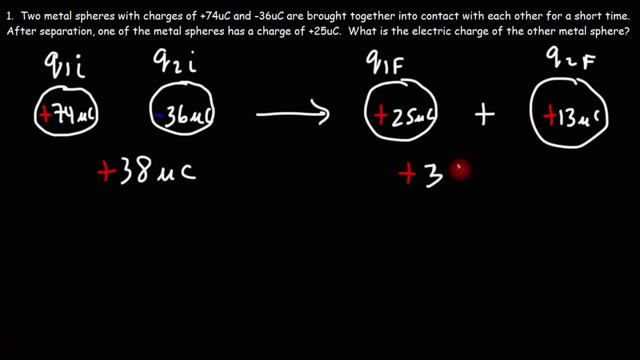 38 micro coulombs. so this is the total charge in the closed system before and after and, as you can see, it doesn't change and that's the basic idea behind the law of conservation of electric charge. the total electric charge in a closed system must remain contact, I mean must remain constant before and after. 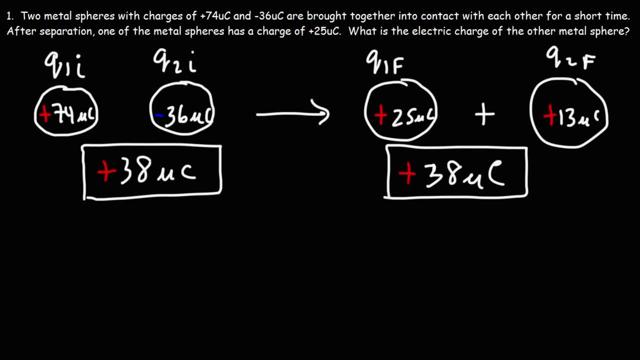 the spheres come in contact with each other. now here's a side question for you: how much electric charge was transferred and from where was it transferred? what would you say? if you want to calculate the amount of electric charge that was transferred from one sphere to another sphere, you need to calculate the change. 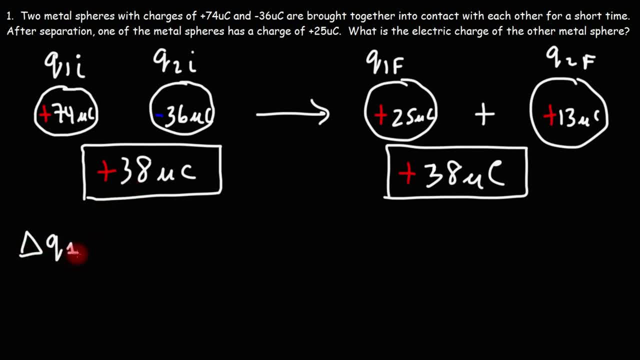 in Q. so let's focus on the change in q1. that is, it's q1 final minus q1 initial. q1 final, that's positive 25 micro coulombs. q1 initial, that's positive 74 micro coulombs. so if we subtract those two numbers, it gives us negative 49 micro. 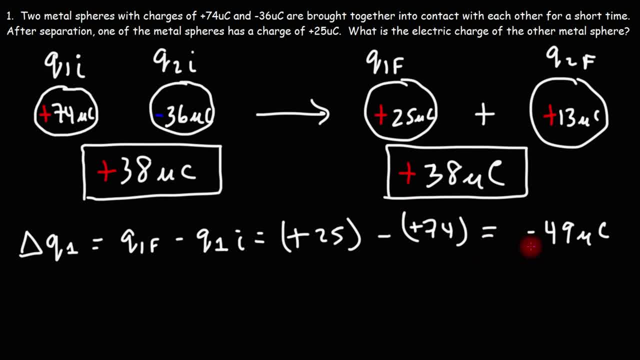 coulombs. now let's do the same thing for the other charge. so delta q2 is going to be the difference between q2 final and q2 initial. so q2 final, that's positive 13 micro coulombs minus q2 initial, which is 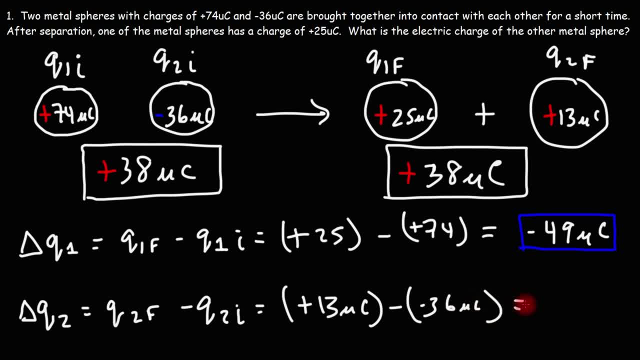 negative 36 micro coulombs. and here we have two negative signs, so this becomes positive, and so we're going to get positive 49 micro coulombs. now this makes sense. if we add these two numbers, the total net change is going to be zero, which also agrees with the law of conservation of electric charge. 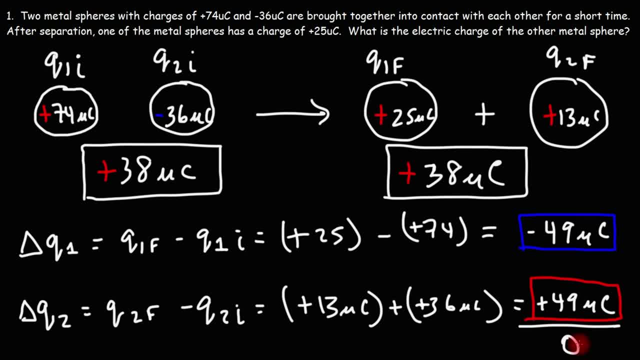 in this case q1. it lost 49 micro coulombs of charge. q2 gained 49 micro coulombs of charge. you contact one metal sphere, it gained positive electric charge and the other metal sphere loss positive electric charge. that's keeping the overall net. 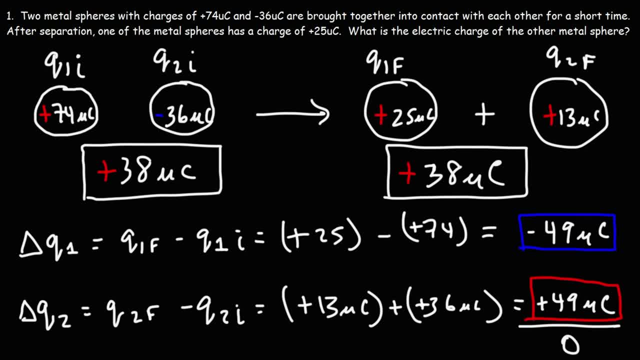 electric charge in this closed system? the same. now. what is the charge carrier here? are we dealing with protons or electrons? what's being transferred? when dealing with metals, electrons are free to move in metals, the protons, they're locked in place. they're fixed in the nucleus of the atoms. so it is the 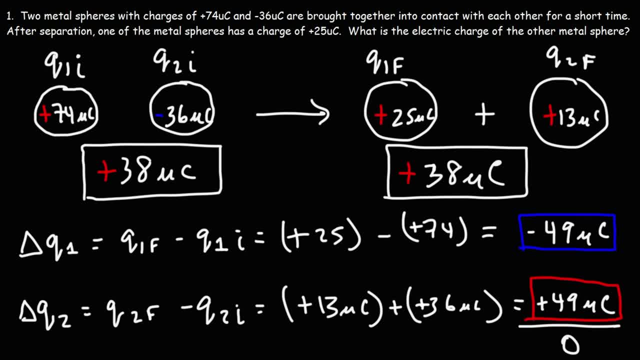 electrons that are being transferred when dealing with metal spheres. so what's going on here? is that negative 49 microcouple of electric charge is negative 49 microcouple of electric charge? is that negative 49 microcouple of electric charge? is that negative 49 microcouple of electric charge? 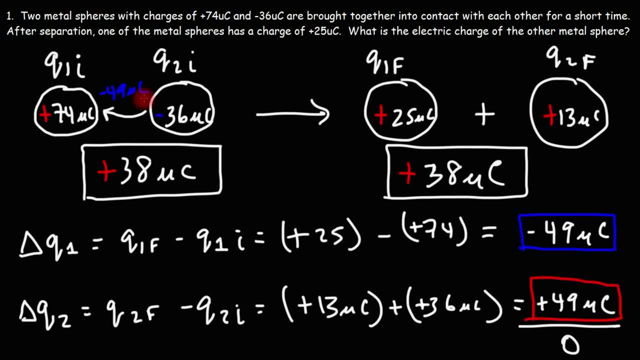 was transferred from q2 to q1. so q1 gained negative 49 microcouples of charge, in the sense that it gained electrons. q2 loss negative electric charge. that's becoming more positive. since it lost electrons, its electric charge will become more positive. it went from negative 36 to positive 13. 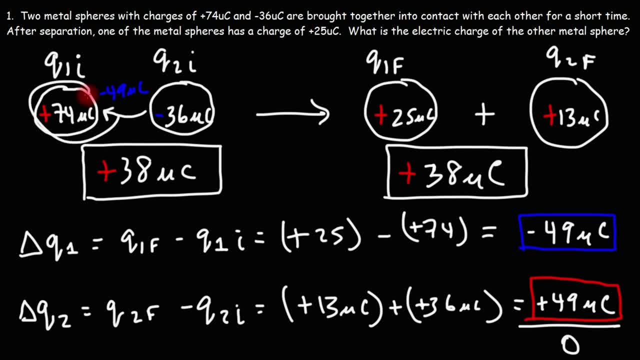 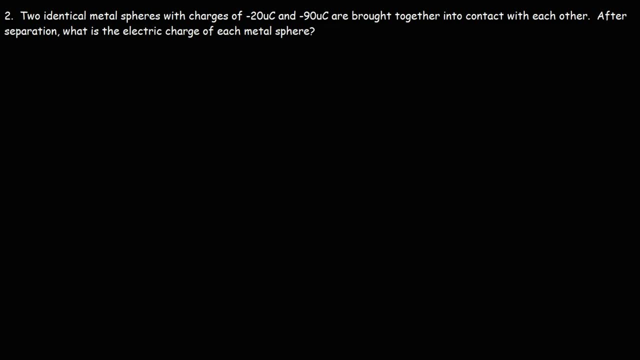 q1 gain electrons. so it became less positive and went from 74 to positive 25, but the total electric charge of the system is constant. now for those of you who want access to more difficult problems associated with electric charge: Coulomb's law, electric fields, electric potential and even electric potential. 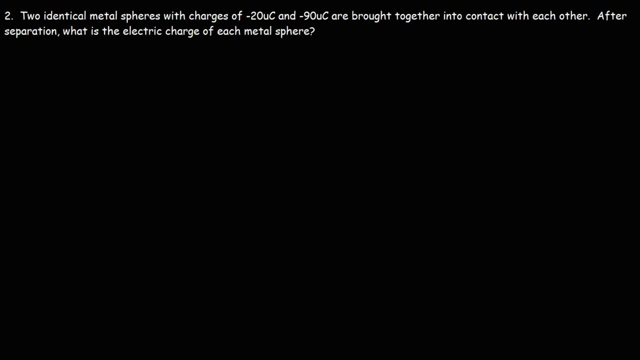 energy and capacitors. feel free to check out the links in the description section below this video when you get a chance, but let's continue to. identical metal spheres with charges of negative 20 microcouples and negative 90 microcouples are brought together into contact with each other. after separation. what is the? 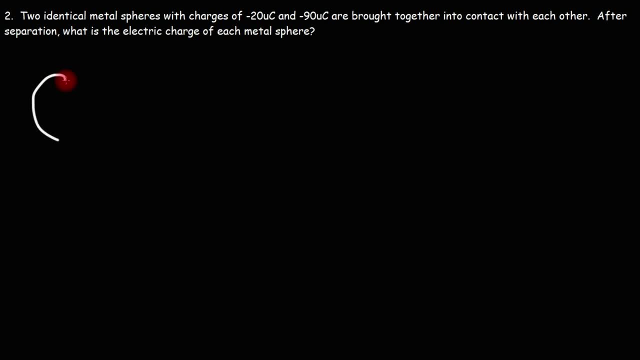 electric charge of each metal sphere. so let's call this q1 initial and you can use the q2 initial. so in both cases we're dealing with negative charges. the first one, it's negative, 20 microcouples. the second one is negative, 90. now keep. 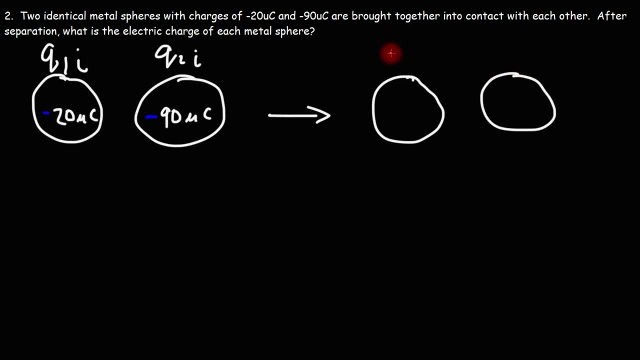 in mind. we're dealing with identical spheres, so this is going to be q1 final and q2 final. now what we can do is we could start with the law of conservation of electric charge. the total charge before contact, Q initial, is going to equal the total charge after. 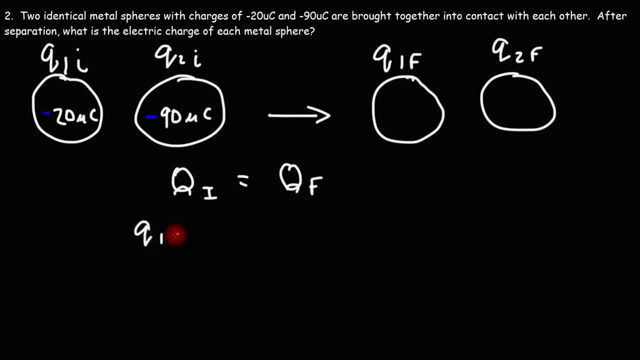 contact Q final. so Q one initial plus Q two initial is going to equal q1 final plus q2 final. now here's what you need to understand with this problem. first, we're dealing with two identical metal means that they have the same amount of surface area. so after contact these: 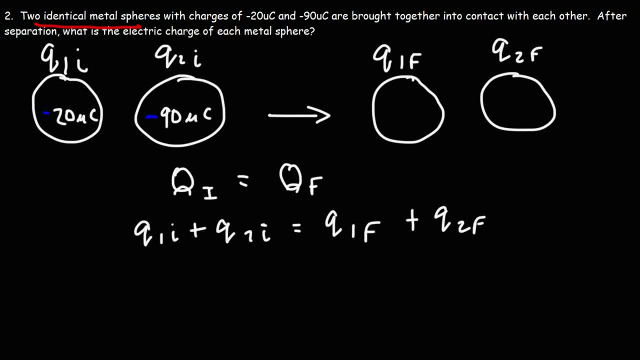 electrons they're going to distribute themselves evenly among the two metal spheres, so they're going to have the same charge after contact. so in other words, actually you just rewrite this here because they're going to have the same charge, q1 final is going to equal to q2 final, so we could just say: 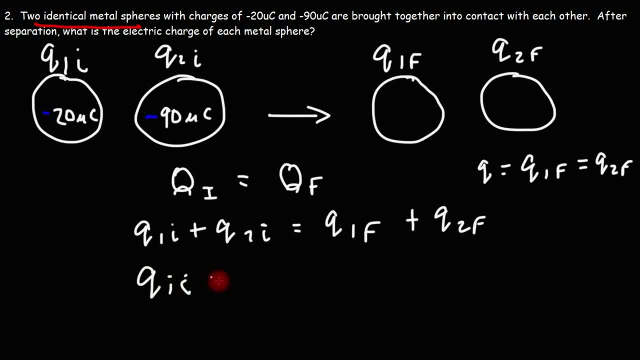 they'll be equal to Q. so we can replace q1 final with Q and q2 final with Q, or in other words, that's going to be Q plus Q, which is 2Q. so now let's solve for Q. so this is negative 20 plus negative 90. that equals 2Q. 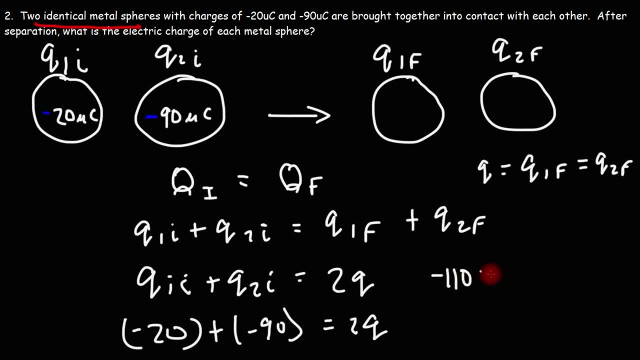 negative 20 plus negative 90 is negative 110 and this is micro columns. so now we just got to divide that by 2. half of that is negative 55. so after contact each of the two charges will have the same charge of negative 55 micro columns. 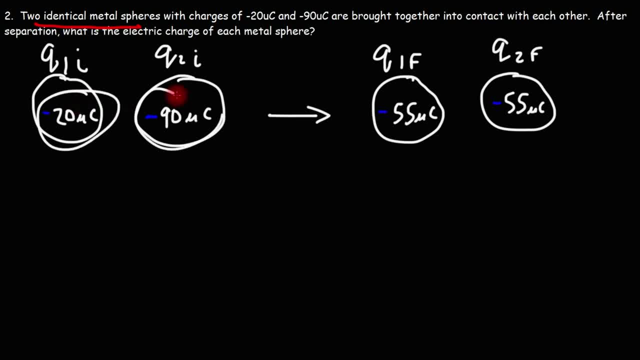 so, as we see in this example, if we add up these two numbers we get a total electric charge of negative 110, and if we add up those two it will be the same. so the net electric charge in this problem is conserved, but after separation each identical metal sphere will have the same charge. so that's the 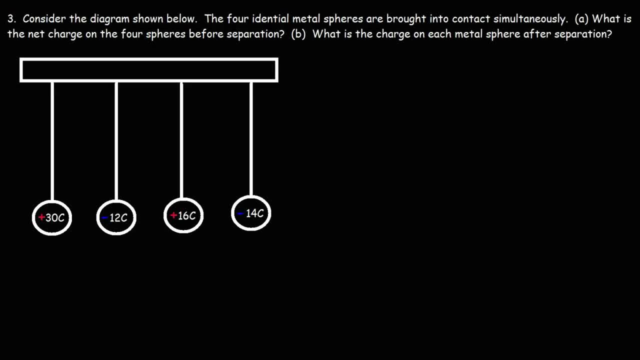 important point of this problem. consider the diagram shown below. the four identical metal spheres are brought into contact simultaneously. what is the net charge on the four spheres for separation? what would you say? let's call this q1, q2, q3 and q4. so we want to find the net charge. 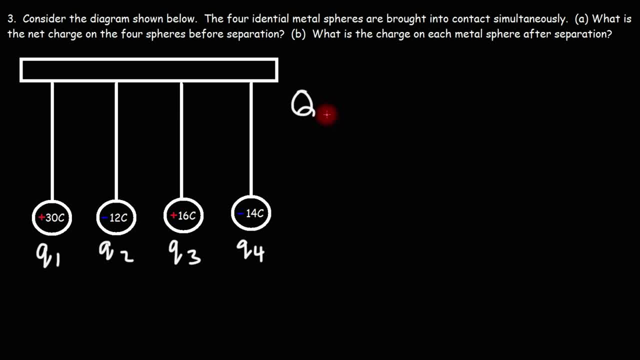 you can also call that the total charge before separation, so we'll call it q initial. this is going to be q1 initial plus q2 initial, plus q3 initial and then plus q4 initial. so what we need to do is simply add up the numbers we have. 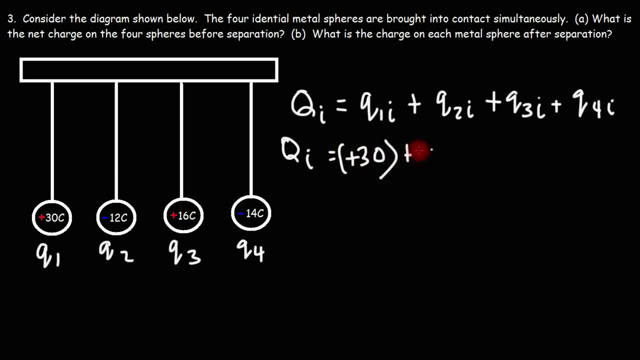 positive 30 plus negative 12, plus positive 16 plus negative 14, 30 plus negative 12, that's 18, and 16 plus negative 14, that's positive 2, so it's 20, so q initial the total charge of the system before separation. but once they are,